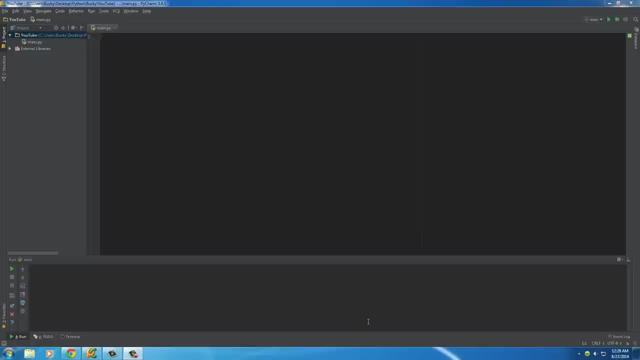 all right, guys, I hope that you're ready to learn about functions, because, oh well, that's what I'm gonna teach you in this video. so if you're not, well, sucks for you. but anyways, what the heck is a function? well, whenever we make a big computer program, that's more than, like you know, these small little samples that. 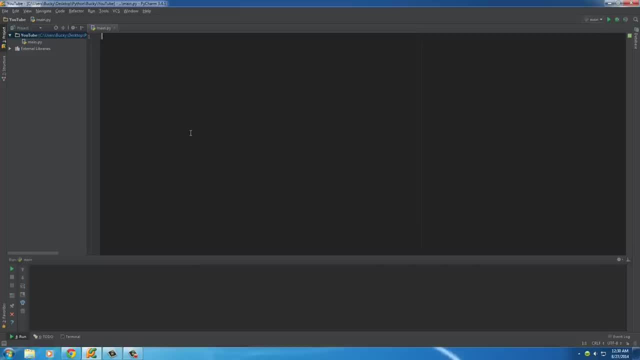 we've been making. it's good to break your program up into manageable chunks. now these chunks are called functions, alright, so it helps organize our program a little bit better. pretty cool, now. another cool thing about a function is what we can do, is we can write a certain bit of code and put it inside a. 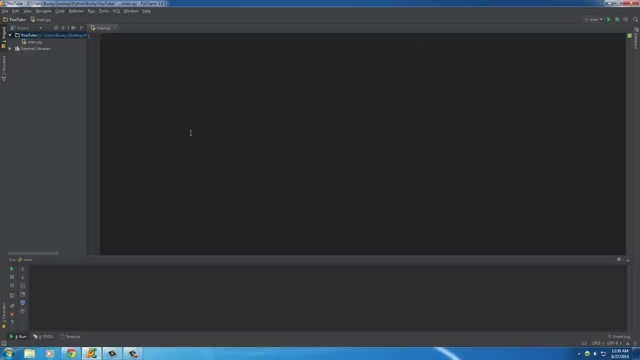 function and then we can use it over and over again whenever we want and however many times you want- really easily. so I'll show you guys how to make a really simple function. right now, whenever you make a function for the first time, write D, E, F. this pretty much means you're defining a function or creating a. 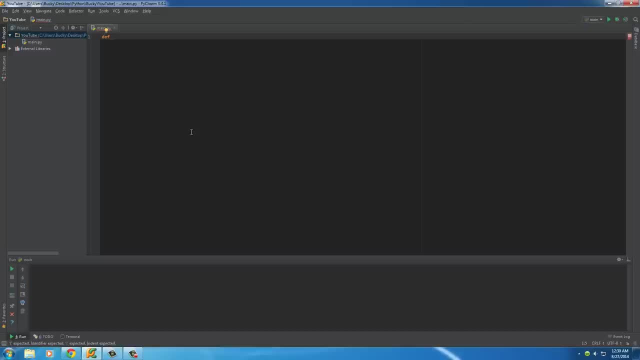 function. now, after this, you have to give your function a name, just like a variable name, and you can name it anything you want. I'll name it beef, because why the heck not? just to show you guys that it doesn't have to be anything special. now, after the name: add: 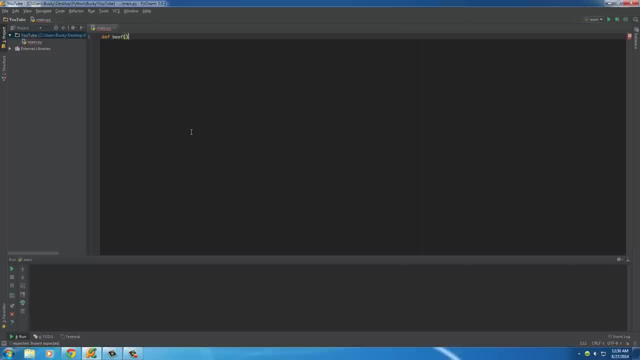 parentheses, and I'll talk to you guys about um what you can use it for later on, but for now we'll just put two empty parentheses and the last thing for your definition is a colon. now, after this colon, hit enter and any line of code that goes in here is going to be part of your function, so any 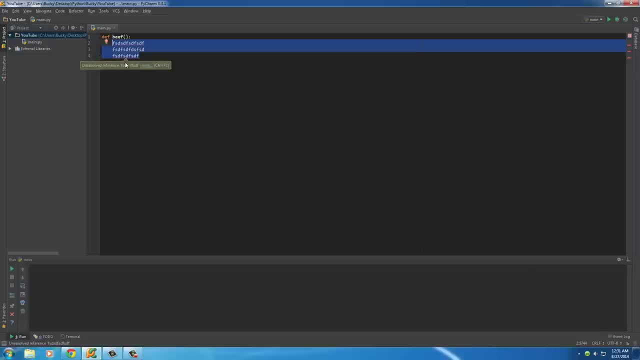 line of code that's inside your function whenever you use it later on. this is the part that executes. so we'll make this a very simple function. print something out and we'll just write. damn functions are cool, alright. so this is a pretty useful function. again, this is just a function called beef and the only job of it is a 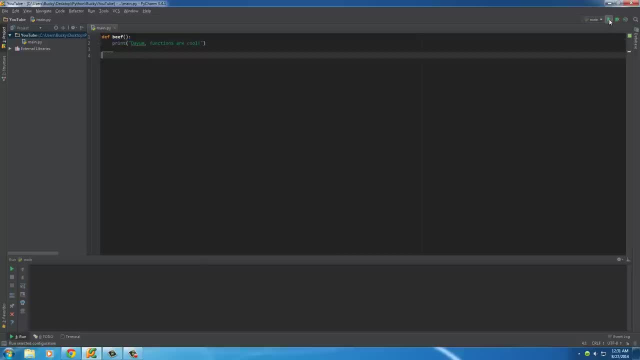 print something out on the screen. so if you run this right now, okay, nothing printed out. it's interesting and the reason for that is this: even though we made a function right now, we didn't tell Python: hey, we actually want to use this function. so whenever you want to actually use the function that you 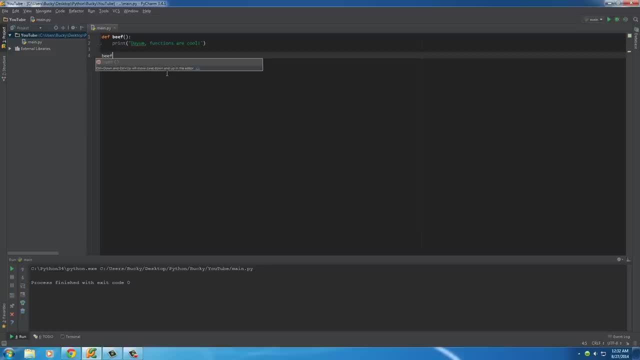 created. what you do is you type the name of your function and then those two little parentheses after. so now, when it gets to this line, it says: okay, use a function called beef. so then it looks for a function called beef, which is this, and it does whatever is inside it. so run it and check it out and, like I said before, the 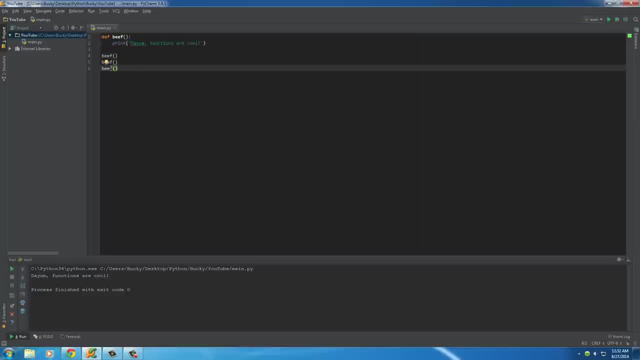 cool thing about these is you can use them over and over and over again as many times as you want. so this we'll call the function. and whenever I say call a function, that's just wait. um, use a function means just a technical, stupid programmer talk calling a. 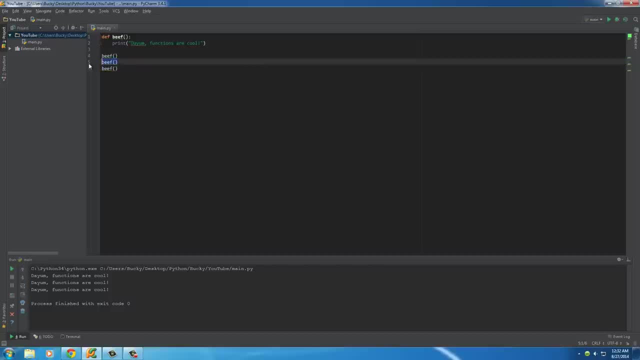 function means using a function, so I'm calling beef three times, simple enough. so now let me show you an actual, useful function, and I also want to talk about what these parentheses are right here. so we'll make a new function. so underneath it myself, a little bit of space. 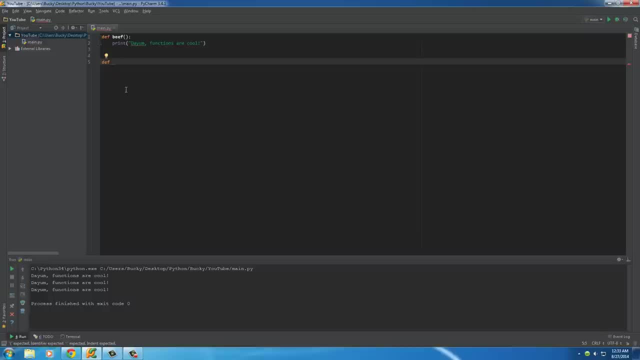 right, new function, of course, def and I'll just write: like a Bitcoin to USD. so what this function is going to do is it's going to take a Bitcoin amount and convert it to US dollars. so if you're curious about like how many Bitcoin, um, like how much one bitcoins worth, this function can do that for you. so, inside, 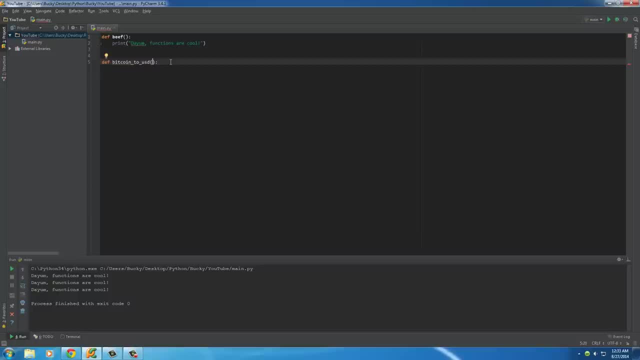 these parentheses right here. whenever your function needs extra information, this is where it goes. so, of course, in order to calculate or convert Bitcoin to US dollars, it needs the value of Bitcoin. do you want to convert one Bitcoin? do you want to convert 10? well, it needs some extra information. so we're 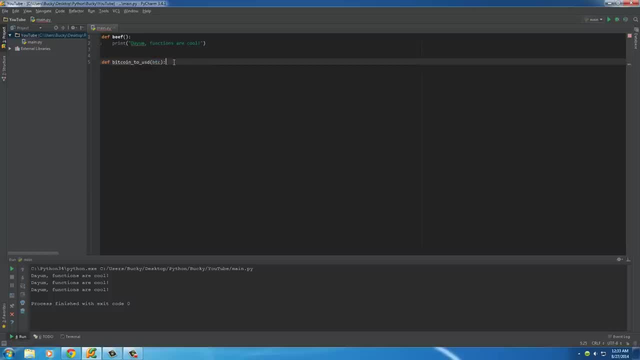 going to throw it in as a variable, and that variable is going to be called B T, C. so now what we need to do is just make um the formula, so we will store the answer in amount and we'll say the amount or the US dollar amount it's equal to is, however,